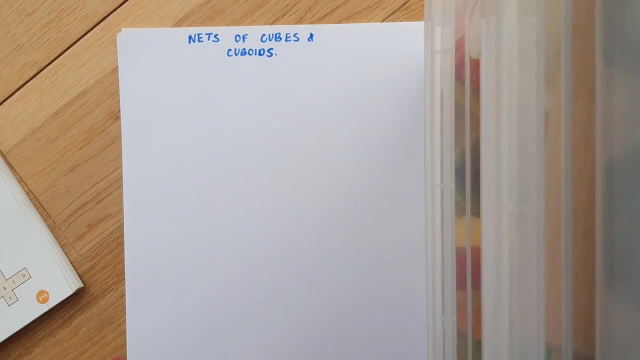 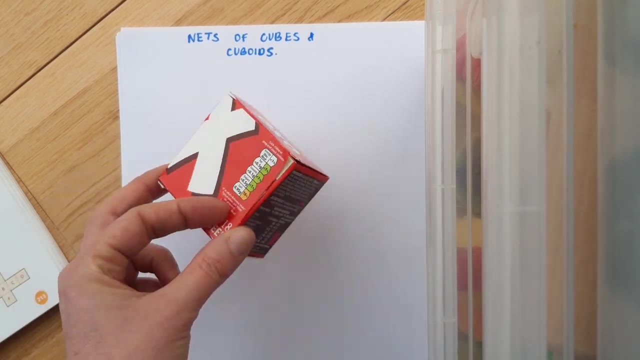 This video is about the nets of cubes and cuboids. So here I have a cuboid box. It's an oxo cube box and you can see that it is a polyhedron. It's a rectangular, solid, and what I can do with a 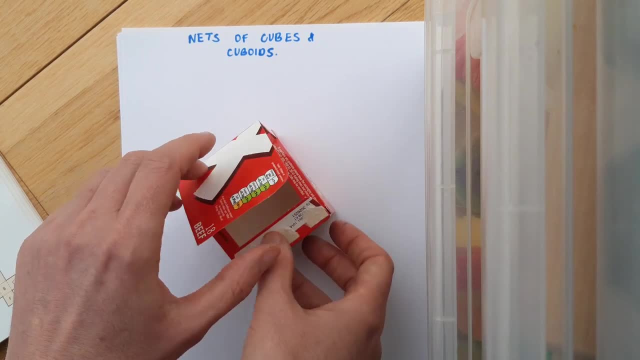 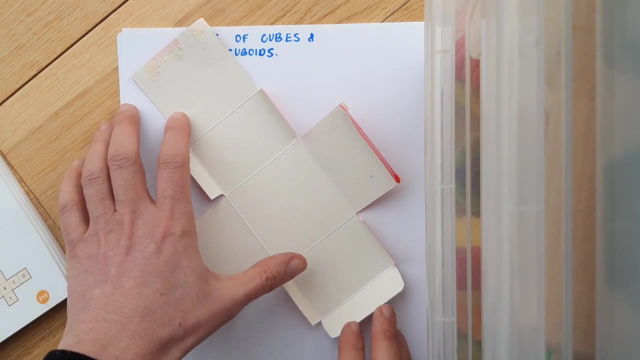 cuboid of this type is, I can actually open it up. So I'm going to open up my cardboard box and I'm going to try and make the net. I've got a few extra bits that I don't really want. I don't. 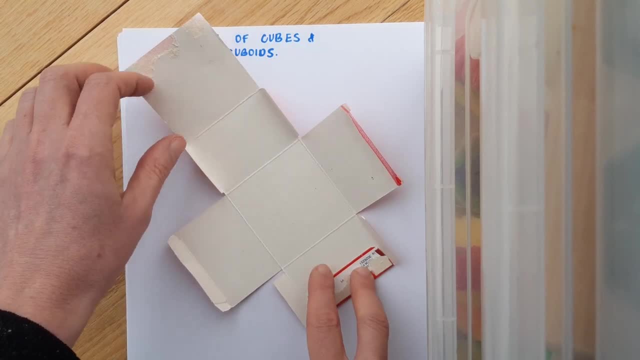 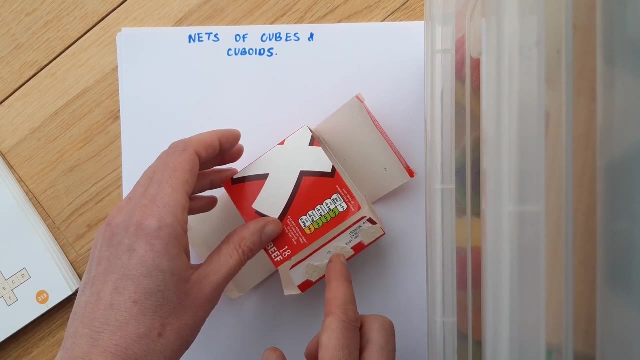 want these flaps that are needed for the box to stay together, but they're not really part of the face. You can see here that if I was to close that back up, this tucks underneath. so it's not part of the face. So I'm going to cut this bit off, this bit off over here and a few more of those flaps. 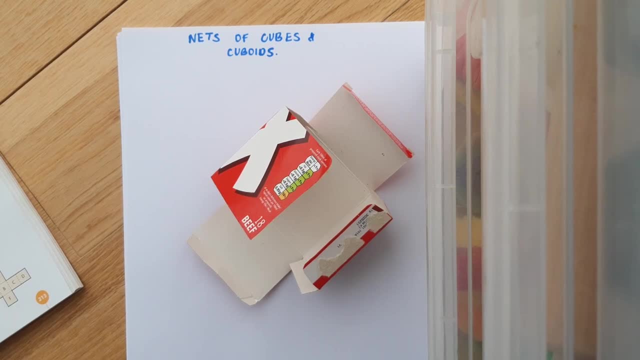 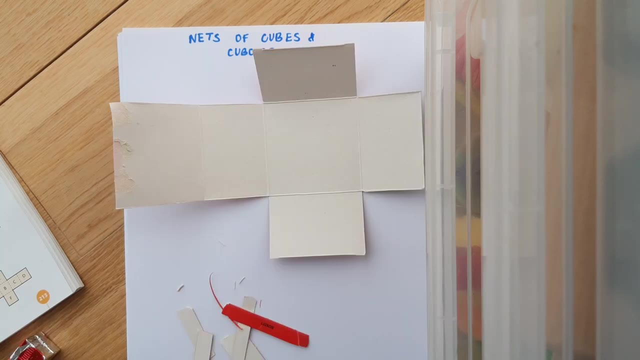 as well. I'd suggest you have a look around the house and see can you find an empty cornflakes box or some little cardboard box that you can chop up in the same way. So I've chopped off these extra little tabs and flaps that hold the box together, and now I'm going to get rid of those. 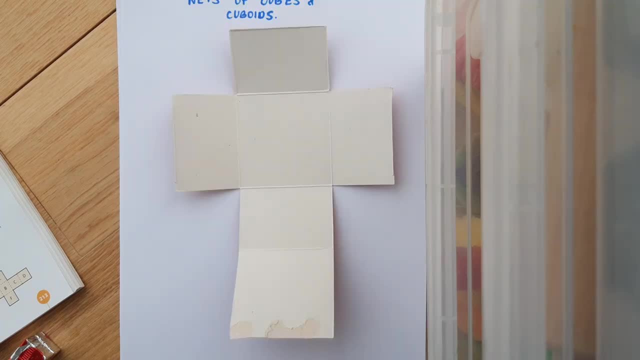 quickly And I'm left with the net of my cardboard box. So the net is just what I have. when I open up the 3D solid, I open up the polyhedron and I flatten it out without any of the bits of tabs and flaps that hold it together as a cardboard box. Just its faces make up the net. 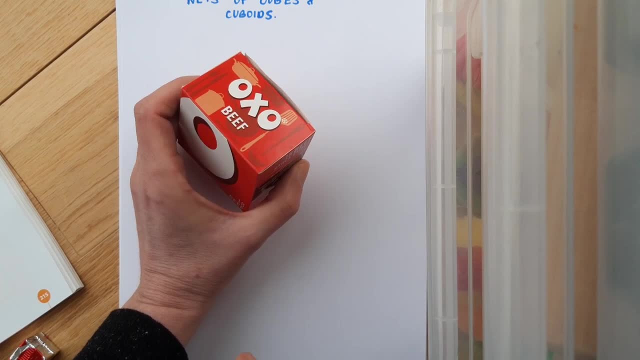 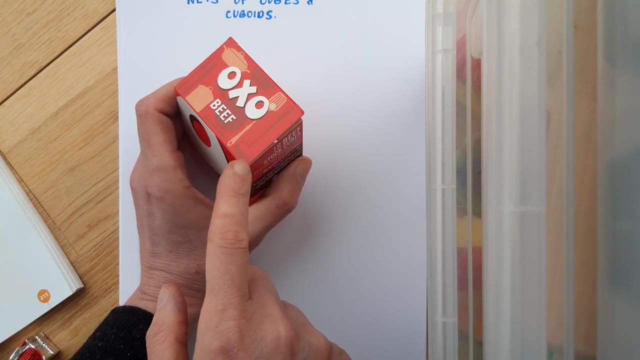 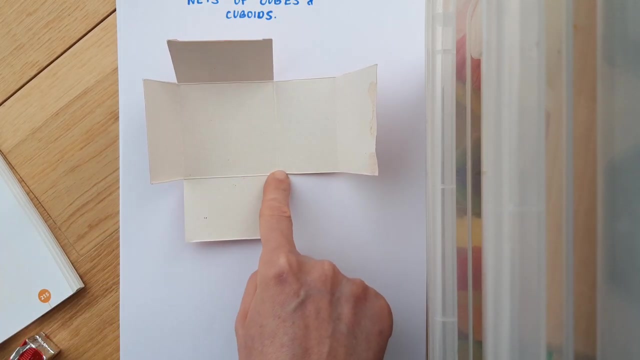 And here I have my closed box again. Now notice, I have my length, my breadth, my height and all of those are coming out of one of the vertices. So if I actually open up my net and I pick a vertex and I draw in the three edges that come from that vertex, I will. 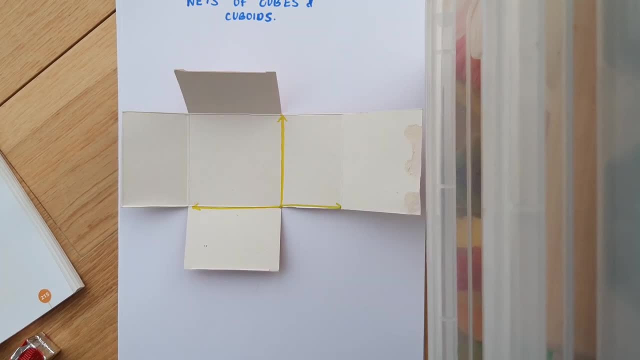 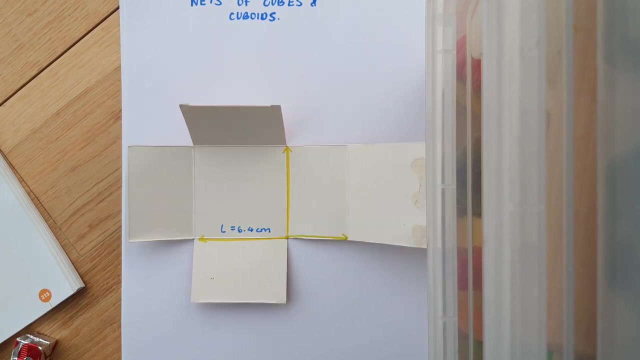 have identified length, breadth and height. I've just marked those in now with a little marker, and to figure out any calculations about my cuboid I'm obviously going to have to first of all measure the length and breadth and height. So I've marked my length in at 6.4 centimeters. 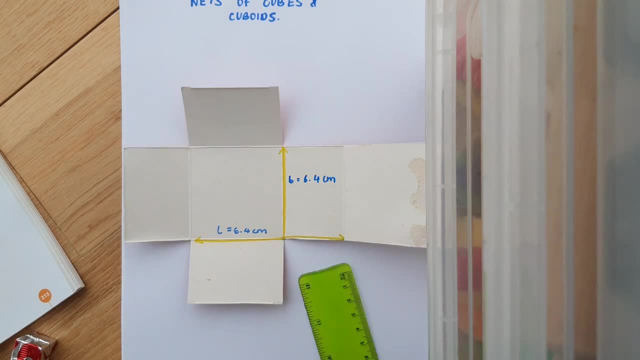 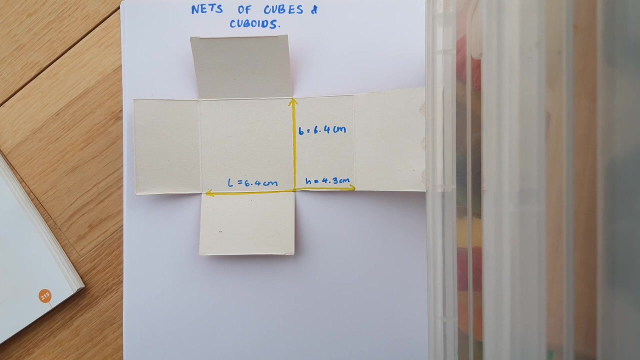 and I've marked my breadth in. that's also 6.4 centimeters, and my height is 4.3 centimeters. So now I have enough information to calculate the volume of the cuboid. So pause the video, work that out and then check your answer. 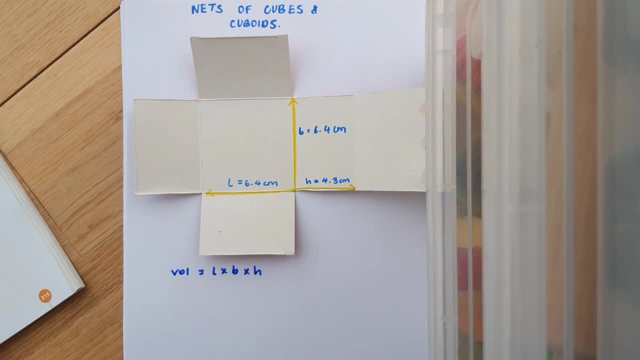 The first thing I want to do is make a note of the formula: length by breadth, by height. So that's 6.4 by 6.4 by 4.3.. Just before you evaluate this, think is there a nicer, more concise way that you could write this? So you could, if you liked, write it as 6.4 squared by 4.3. 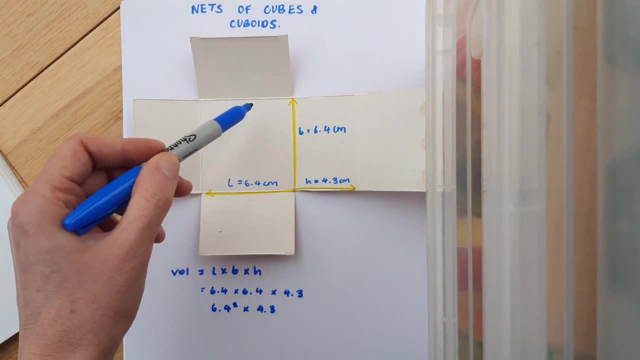 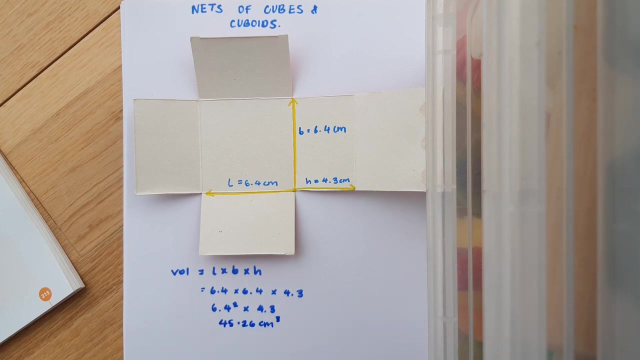 and that gets across the idea, of course, that one of the faces is square. That's reflected there in the square in the calculation. So my volume comes out as 45.26 centimeters cubed. I can also calculate surface area using the same formula as before, and it's: 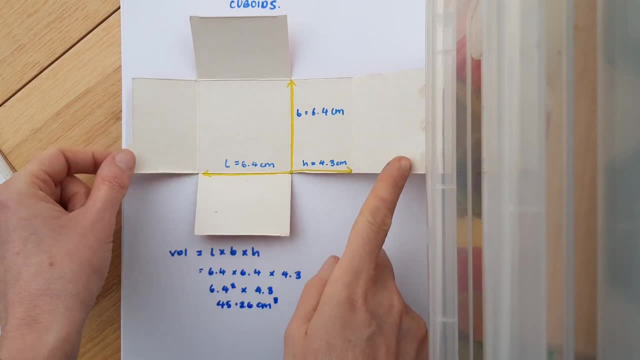 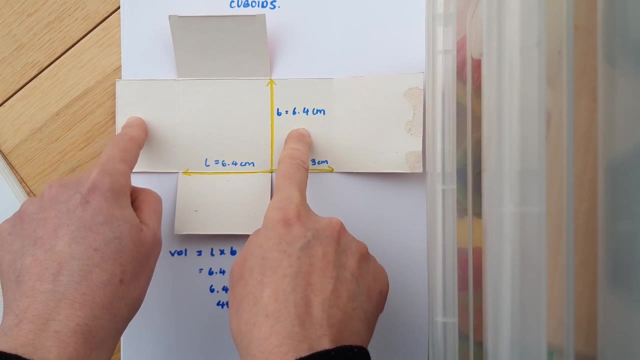 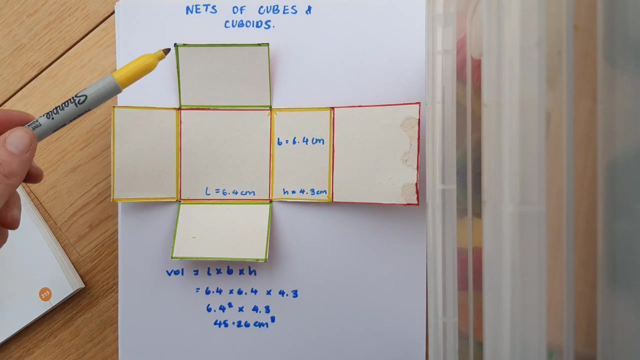 nice just here to have a bit of a visual reference as well. Of course I can see that I've got these two faces equal in area and these two faces equal in area and these two faces equal in area. So just for clarity there, I've highlighted top and bottom in green, these two sides in yellow. 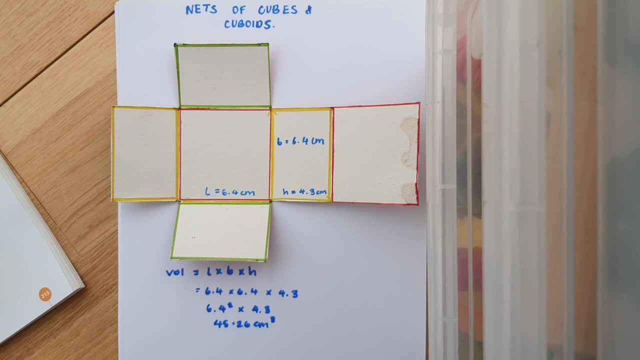 and these two sides in green. So I've got these two sides in yellow and these two sides in green. So when I want to calculate the surface area, of course I'm going to be saying length by breadth, which is this guy, by two, to include this face also, Breath by height, which is 6.4 by 4.3 by two. 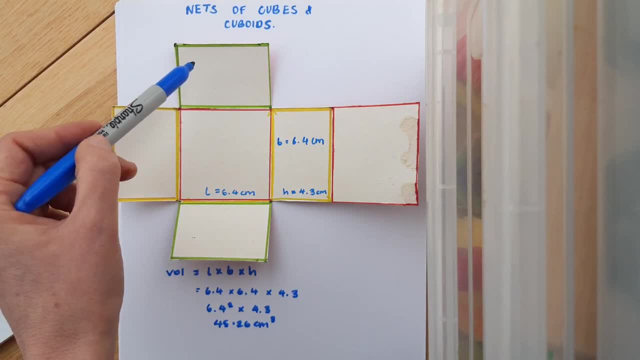 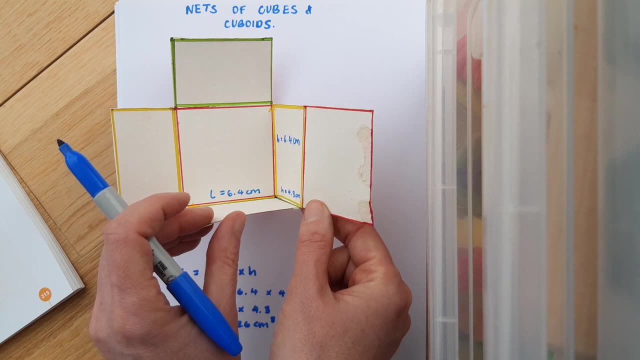 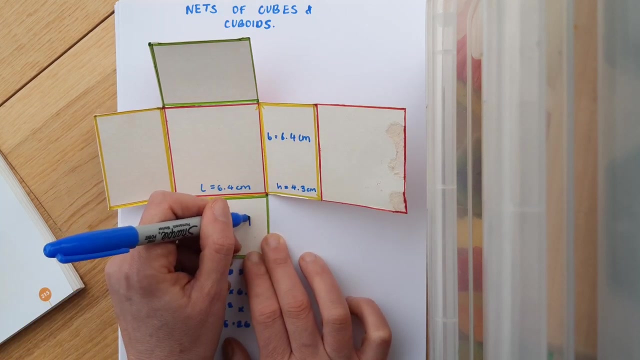 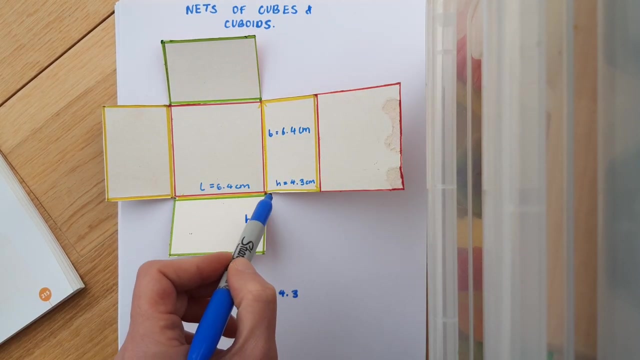 and then, of course, I'm going to also have. well, I wonder what the measurements are here. Notice how, when I fold these two up, they're the same measurements, Because the box has to fit together. so this measurement here is the same as this measurement here, and if I ever have two edges meeting at a right angle, 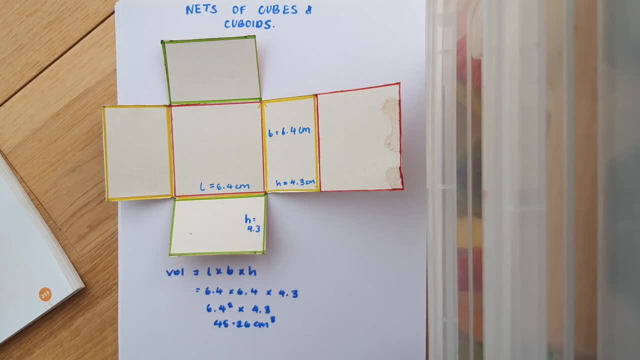 they'll always be equal in length like that, especially if it's an open section between them. so I'm gonna have 4.3 and 4.3. so it's gonna be this face is length by height, and there's two of those also. I can actually write the calculation into the calculator and write it down here in the 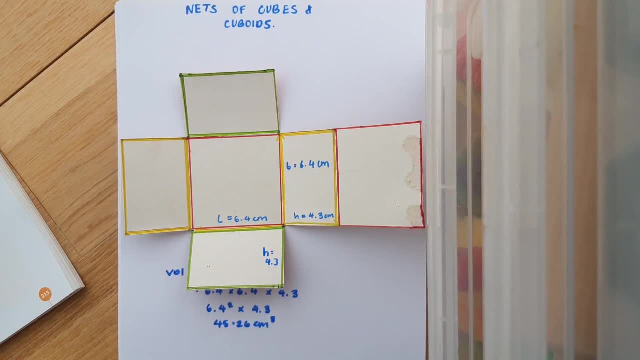 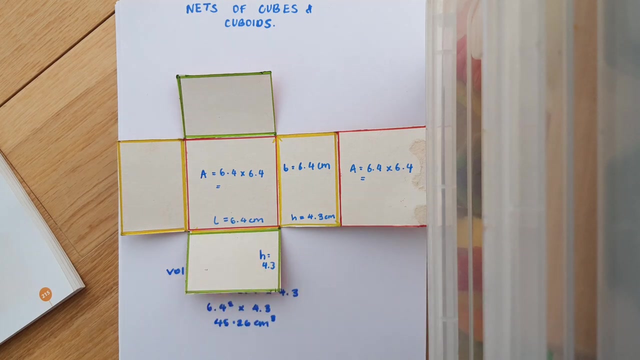 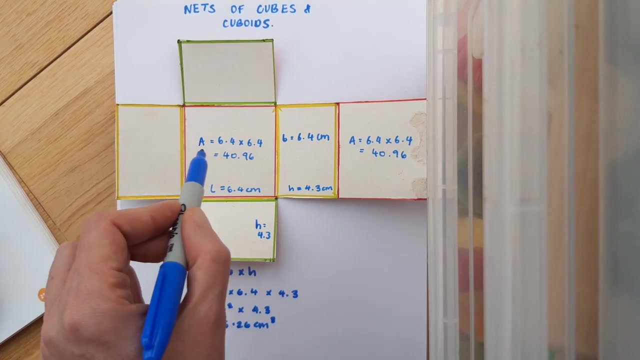 calculations onto my net, and if you've done your own cardboard box net well, then you do your calculations for the area of each individual face onto your net as well. so, for example, each of these faces is 6.4 by 6.4, so each of those faces is 40.96. now I'm going to do the yellow faces here and here. 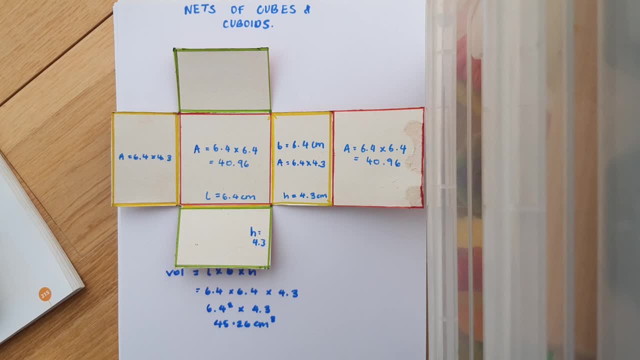 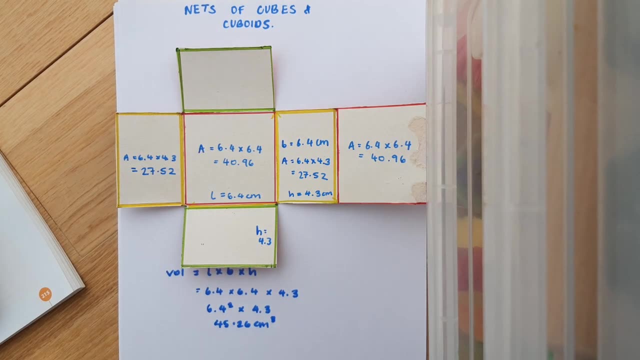 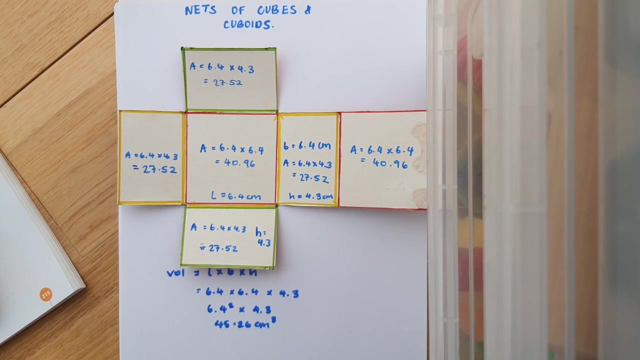 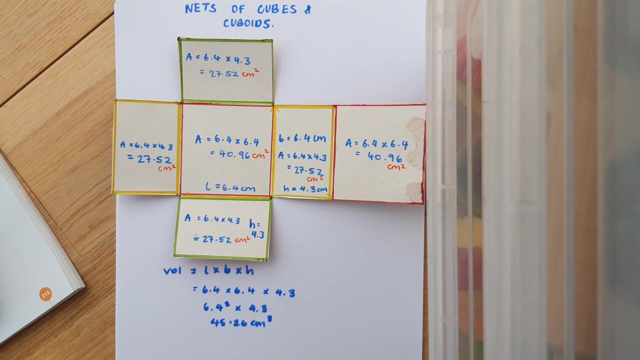 and each of these comes out as 27.52. and finally, I'm going to do these green faces, and they're going to come out as 27.52. also, don't forget, I need my units, of course, for each of these and in each case they're centimetres squared, because my original measurements were in. 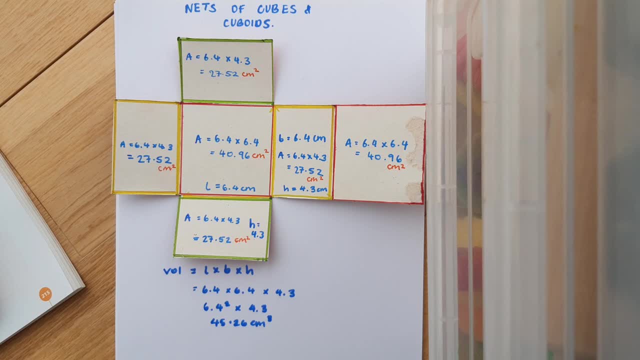 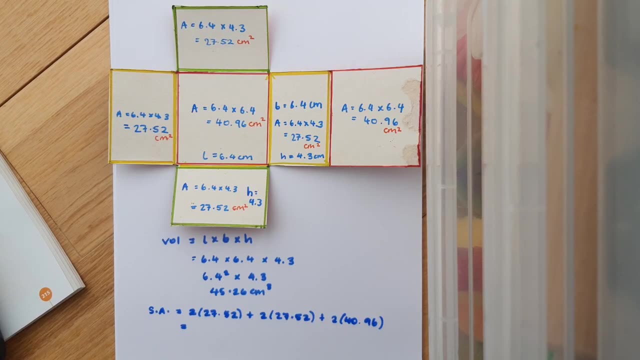 centimetres, and area is always centimetres squared to get the same result. so I'm going to my total surface area, then I'm simply going to add up each of these and my answer finally comes out as 192 centimetres squared. If I had calculated this using the formula, I would of course have got 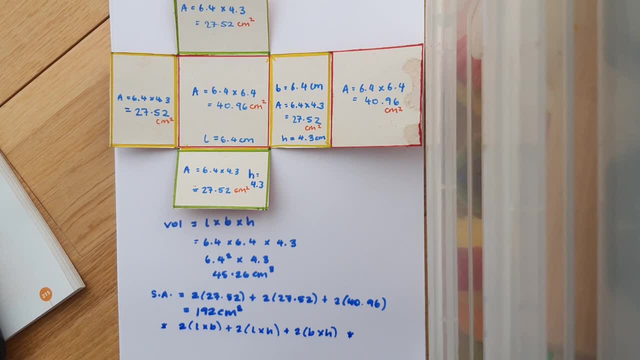 the same answer, but we're just simply representing it visually here, so we can really see what's going on Now. having glanced back at my calculator from a little bit earlier, I've just spotted that I've made one calculation error in this video. I want you to pause the video at this stage and see can. 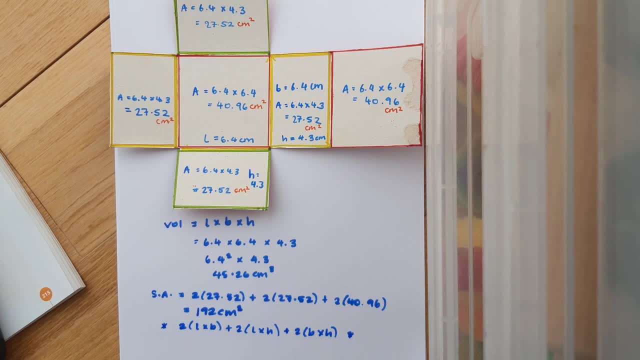 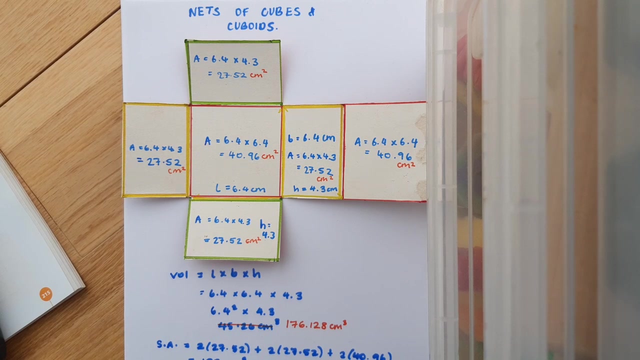 you find that calculation error? maybe you've already noticed it and correct it. So have you found it? Well, it was actually here. in my volume That answer should have been 176.128 centimetres. Sometimes I can be asked to draw the net of cuboid, in which case I have to make sure to use a ruler. 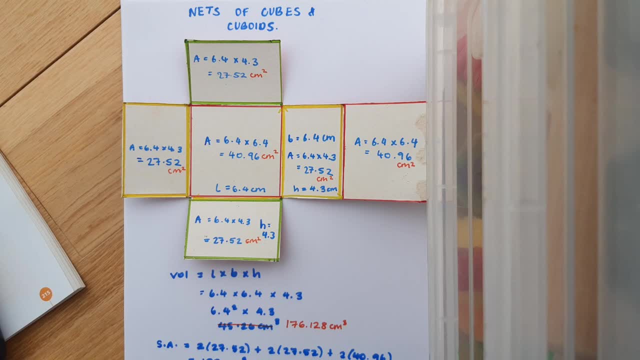 in order to get nice straight lines and get all my measurements as accurate as I possibly can. So what I'd like you to do now is have a look at the information in this diagram and, on a fresh page, I'd like you to draw out accurately the net of this cuboid. 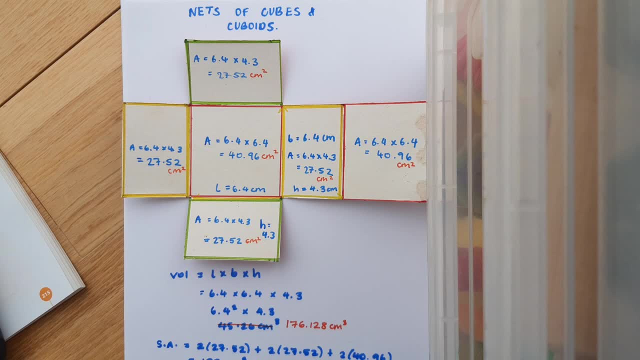 Pause the video here so that you've got access to the dimensions, the measurements, and then I'll show you how to do that. And then I'll draw mine and unpause and we'll see if we have the same thing at the end.